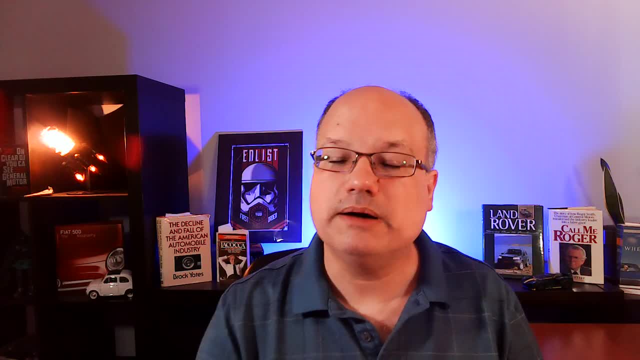 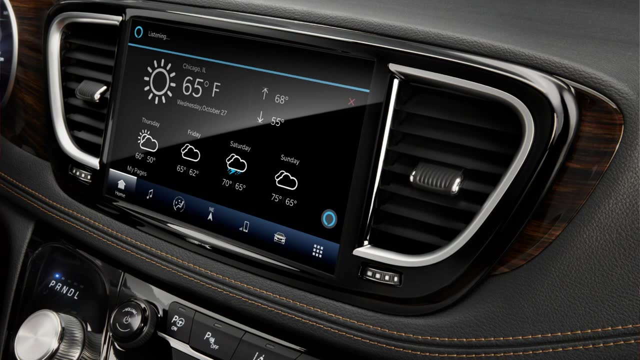 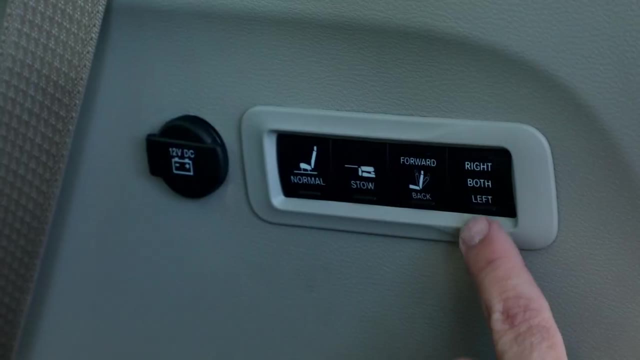 style. It is subjective. modestly attractive, Active outside, a modestly attractive inside. Their Uconnect system- probably the best in the market. honestly, Stone goes seating on the non-hybrid models and yes, that means they have a hybrid option which gives fantastic gas mileage, but you pay for it. The problem with the 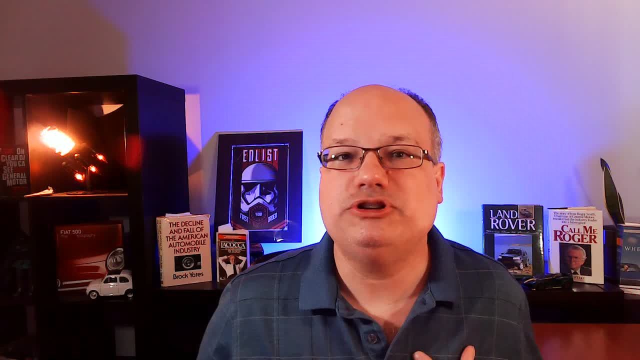 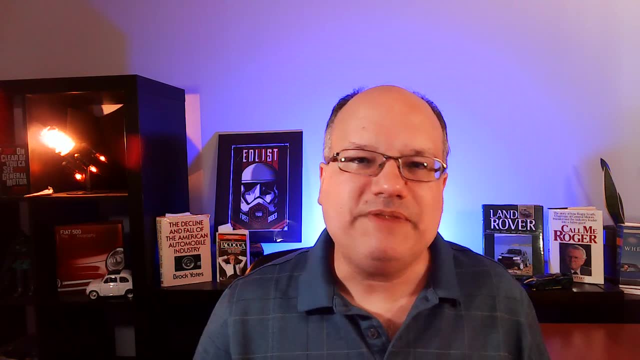 Chrysler is really, really simple. It boils down to two things. The first is styling. While this is subjective and you may disagree with me, but the Chrysler is really really simple, I find it a little awkward. It's weird to me that the company that innovated minivans for so many 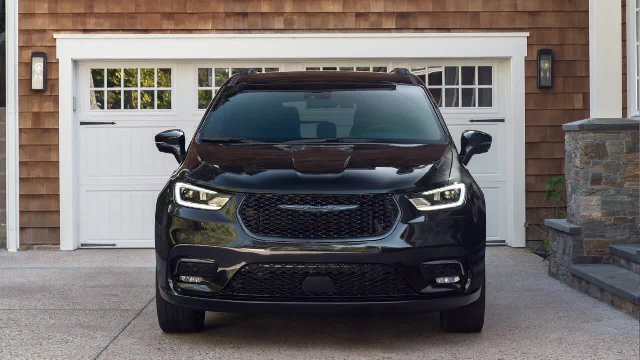 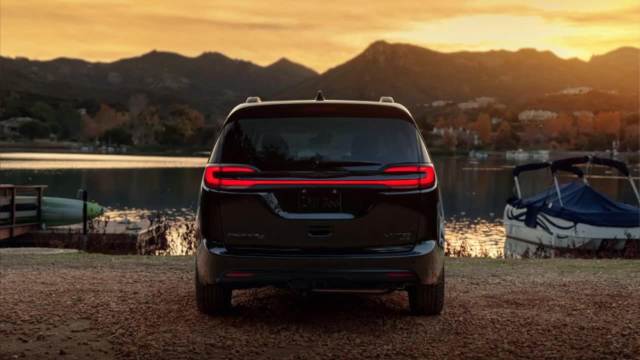 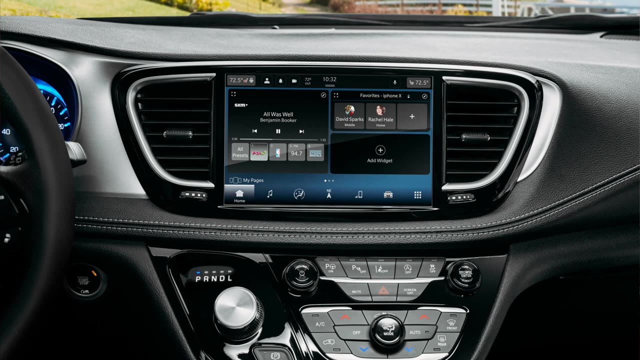 decades has ended up with something that seems a little bug-eyed, a little narrow, a little tall. It's just a little awkward. overall, I think the interior is attractive, but some of the materials aren't quite there. It ends up being somewhat compelling, but not necessarily for the price. 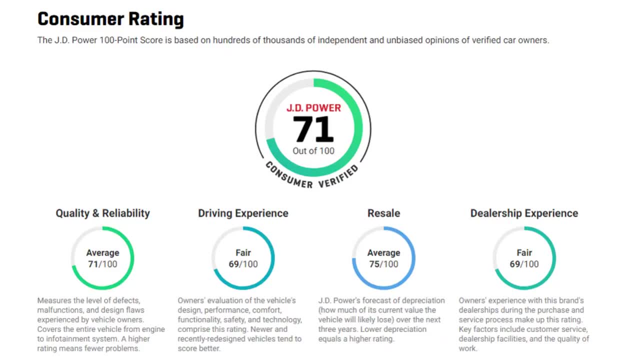 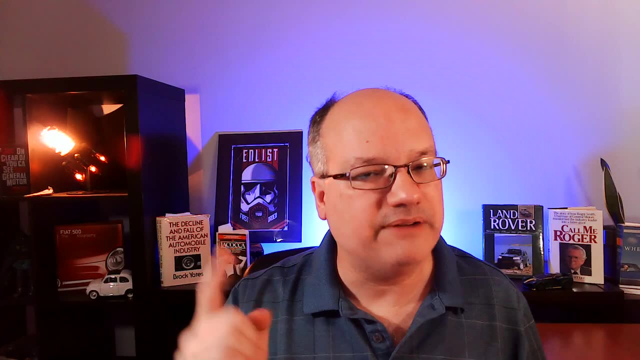 What kills it for me is the reliability. The Chrysler minivans are not reliable overall. Now, of course, I'm going to hear from people who say I've had one, it's been flawless. but I have talked, read and heard people who absolutely they're miserably unreliable and unfortunately a lot of it comes from the engine. For that reason I would leave them to one side. I think the Chrysler the Pacifica is a little long in the tooth. I think Chrysler missed the mark with it. 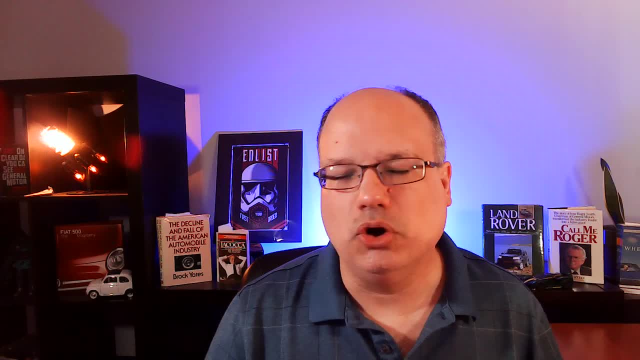 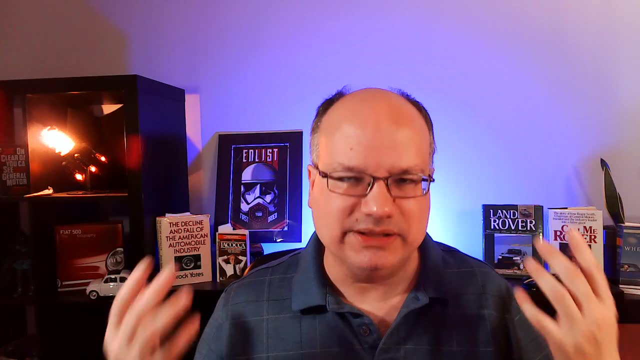 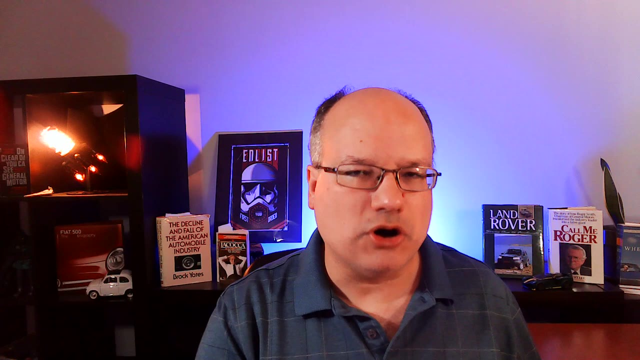 And I just think they let it languish on the vine a little too long. That leads me to number three, the Kia Carnival. Now, once you get over the ridiculous name of this vehicle, I'm surprised that Kia stayed in the minivan market. Their earliest offerings were: 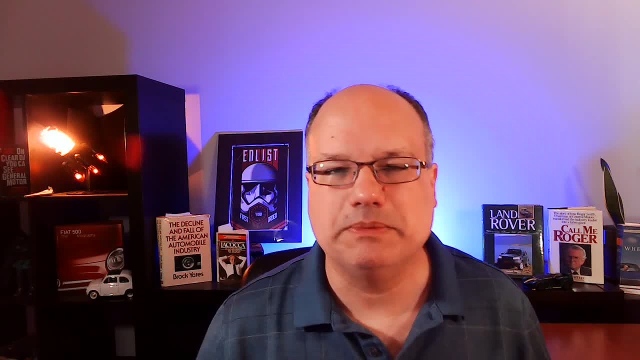 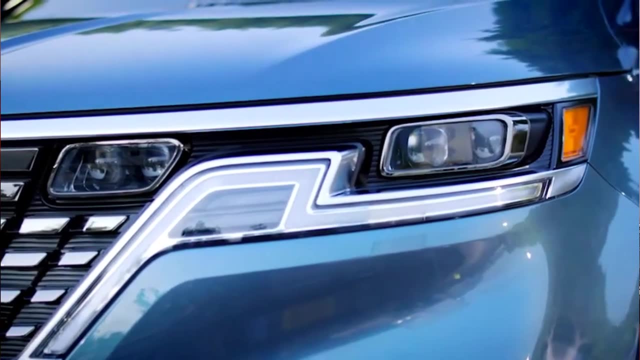 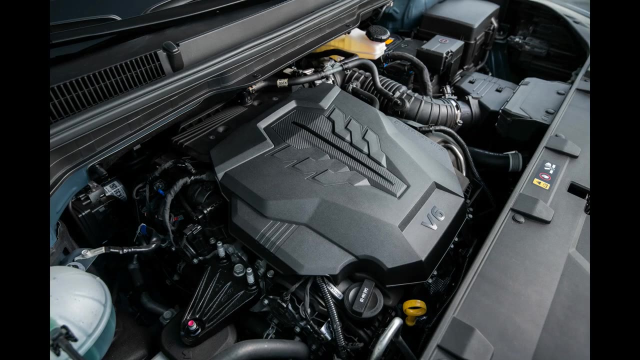 okay, but not exceptional. I guess they sold enough to make some money off of it And what they came out with is something that they intended to look a little more SUV-ish, to take some of that stigma Of owning a minivan away And they come out with a very compelling package It has. 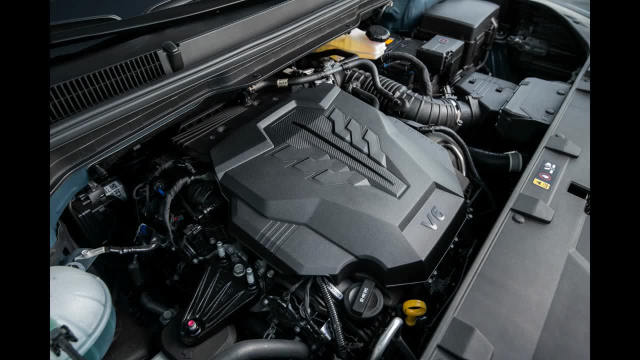 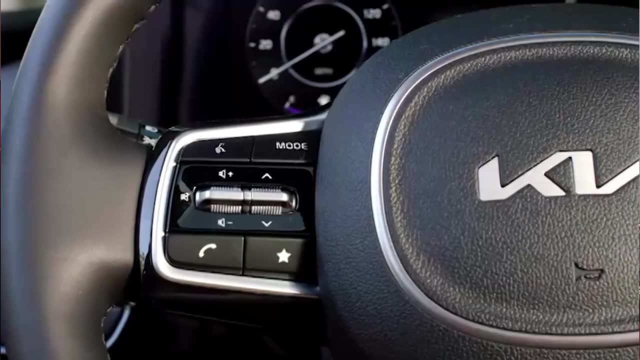 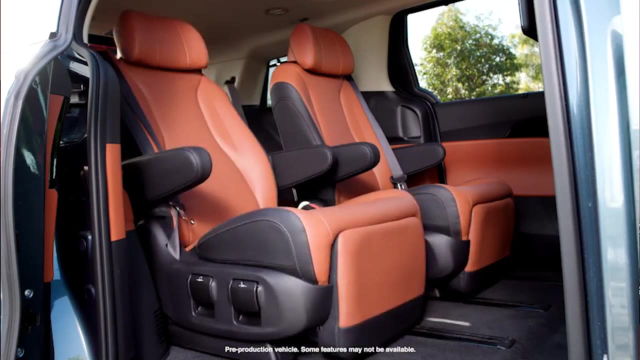 believe the most powerful engine- V6, in the minivan market. It's got a really good looking interior. it links in pictures that you know is reminiscent of some of the bigger SUVs that they do And it's fully competitive in the market And I think parts of its angles look really 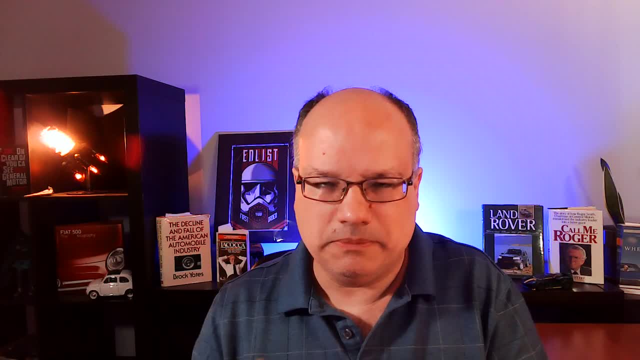 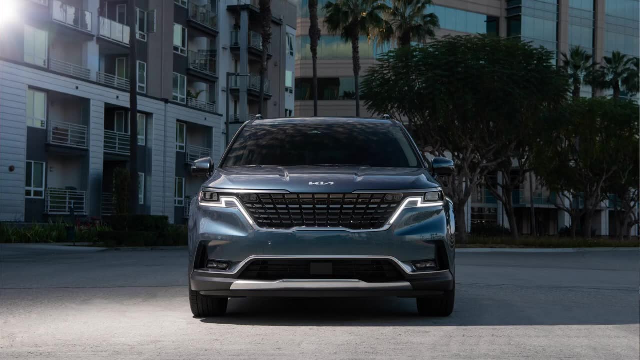 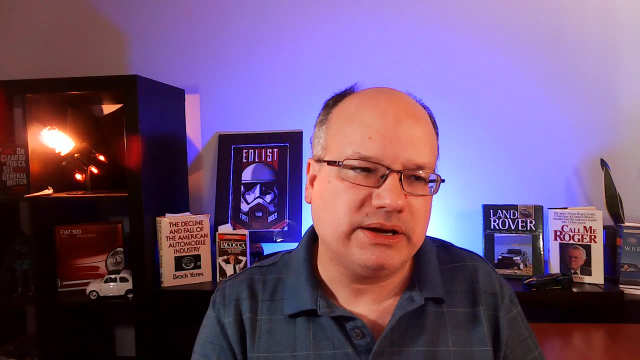 really good. But overall the argument against the Carnival- if you can get over that ridiculous name- is, how is it better than the top two? And the fact is is it's not. It just ends up being a little bit more like. 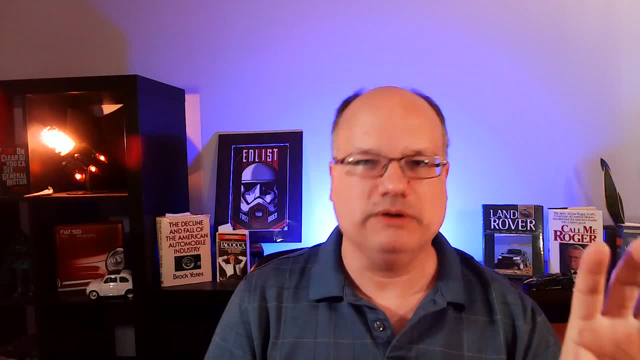 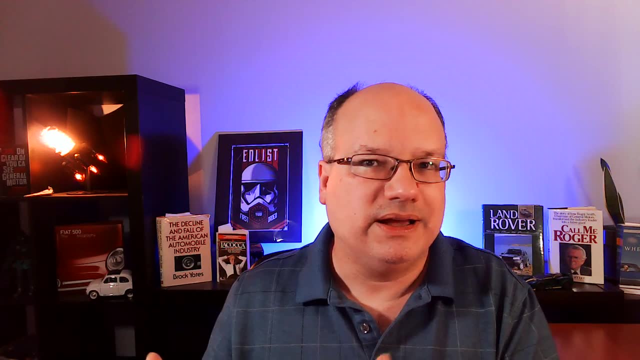 Kia took an old Dodge Caravan and then said: how can we make this better than taking, say, an Odyssey and trying to improve on it? The Carnival's not bad, don't get me wrong. And I truly will say right now: 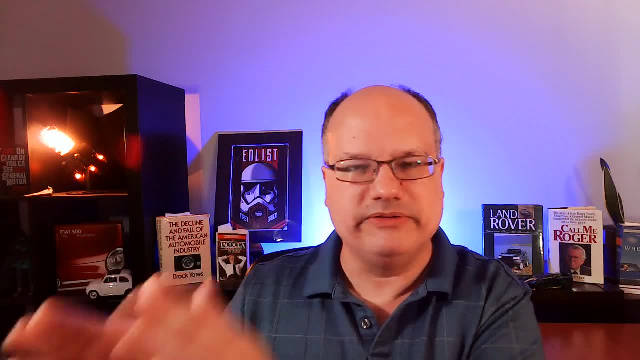 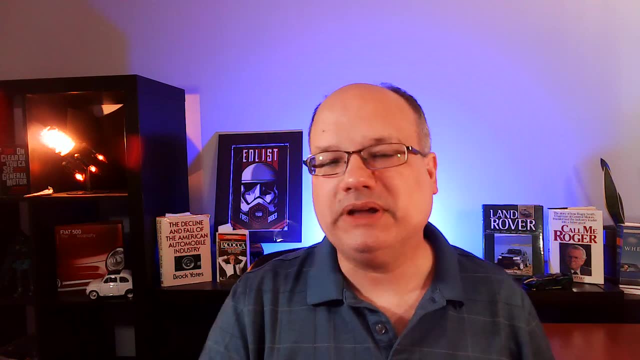 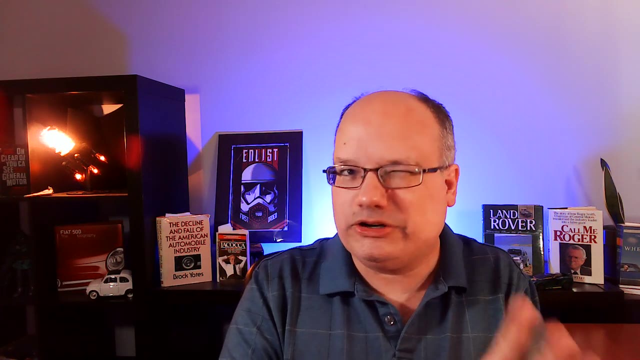 if you're in the minivan market, drive every single one of these, See which one fits your needs, See which one the price for the equipment works for you. And if you pick the Carnival, I totally understand. I think it's an okay looking vehicle with an pretty darn good looking interior, and 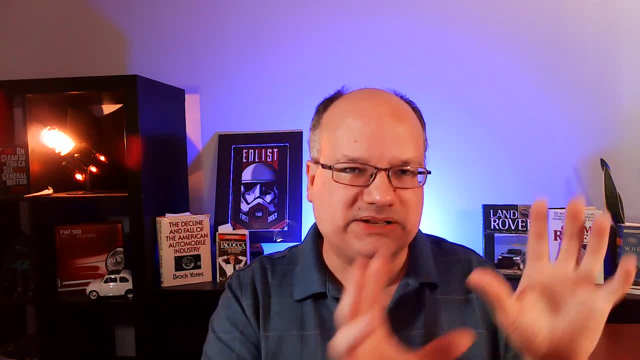 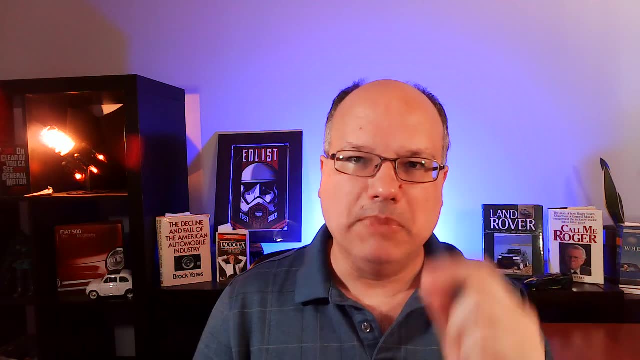 enough flexibility, But I don't think they took the best of the best and tried to beat it. I think they actually took an older Caravan and updated it to the modern day much more than Chrysler did, who went off on some tangent with 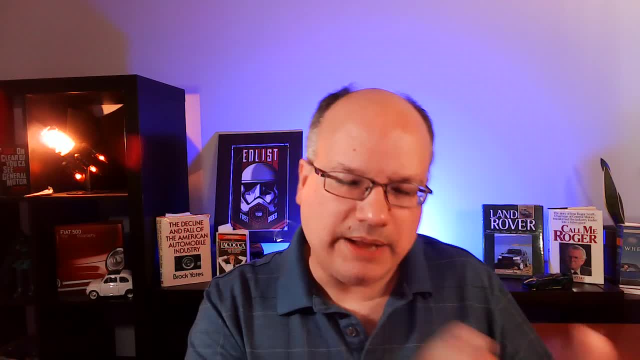 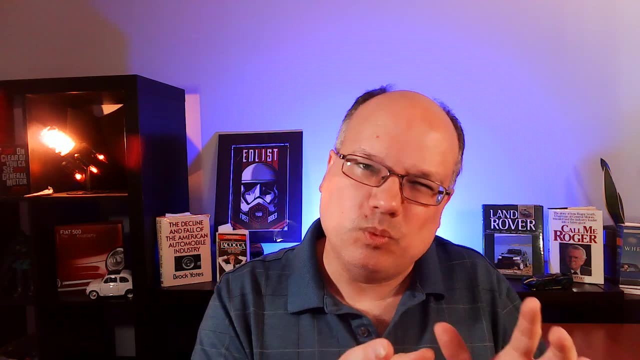 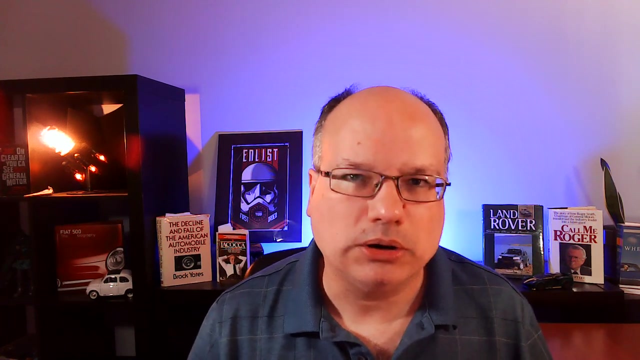 their styling. Carnival's a good option. If the reliability, if it holds up, it's a really good option. But it's not a huge discount. And why would you choose it over one of the top two? Now for the top two. don't be surprised who these two are, but I've got to give number two to the. 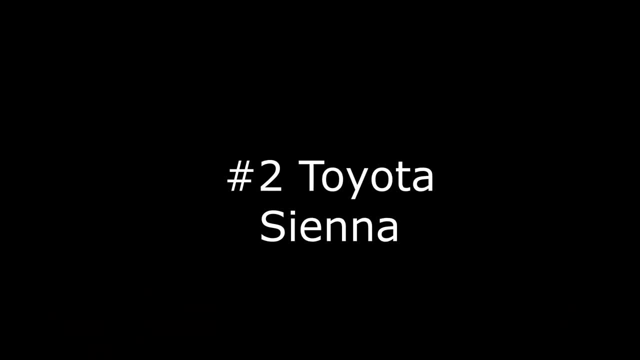 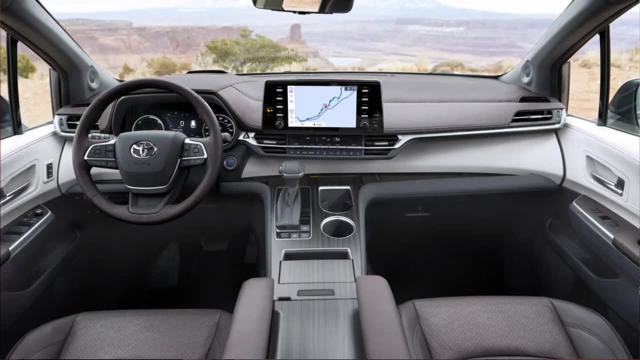 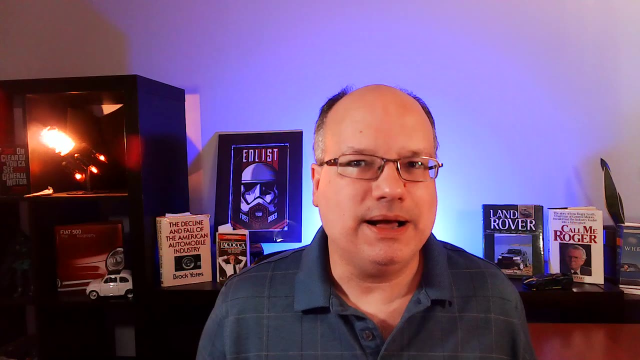 Toyota Sienna. Now here's the thing is. I really like the Sienna. It is really good looking outside, It's really good looking inside And I'm kind of impressed. they only offer one powertrain option, That is, a four-cylinder hybrid. It's not an option, And so here you get a hybrid, whereas the Chrysler Pacifica starts at like $15,000 extra. Here you get it standard with the Sienna. It's a strong seller, It's at Toyota Reliability, it's super comfortable, It's flexible. I think there's almost nothing not to like about this. 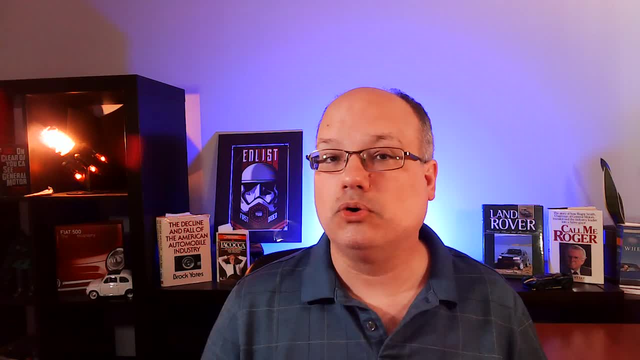 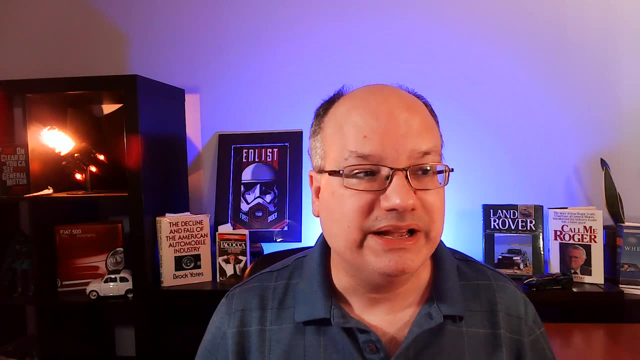 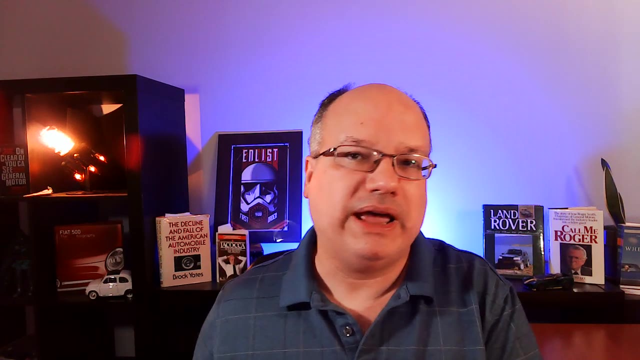 minivan And I understand if you buy it over, say, the Carnival or my number one choice. I looked at the Sienna multiple times and thought, yeah, this is the one I want, And then changed my mind later on. It's a solid, solid entry from Toyota and expected Toyota. 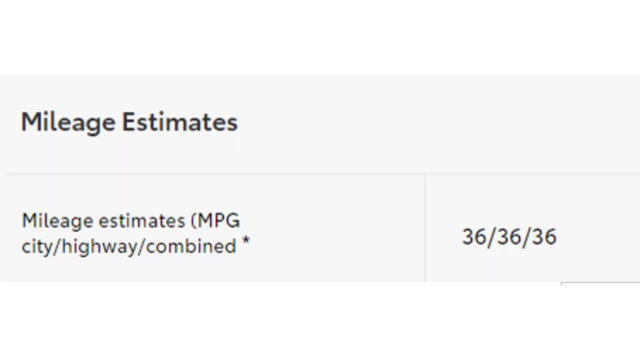 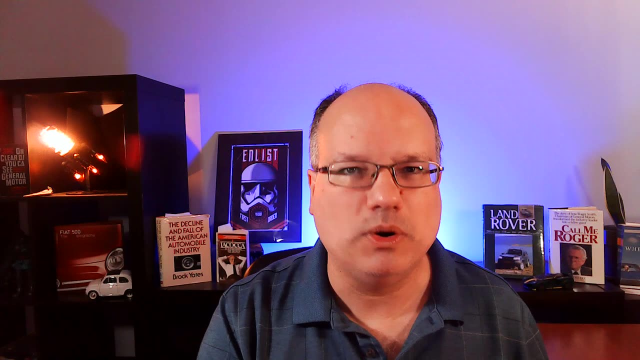 Reliability, And that hybrid powertrain gives fantastic, fantastic, fantastic, fantastic gas mileage. I think it's a strong contender. It's nearly number one, which is why I say number one could be a tie, But ultimately I've got to go with my number one being the Honda Odyssey. 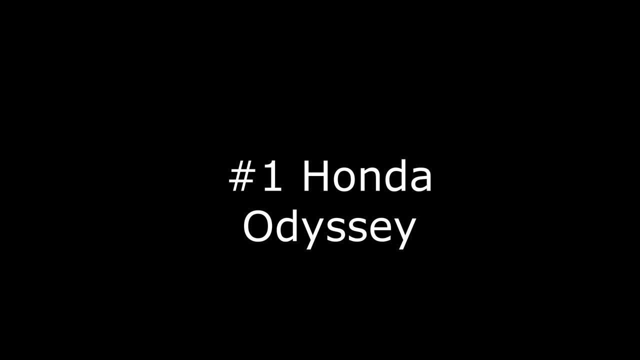 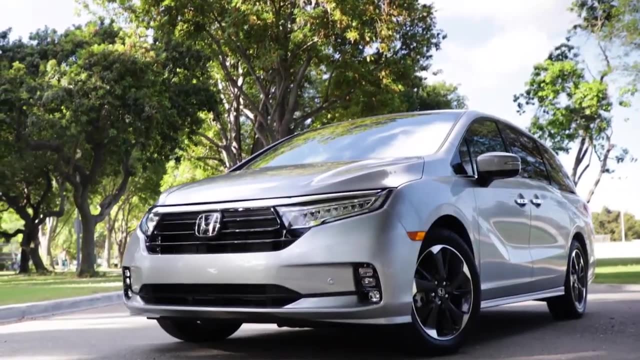 There's very little to dislike about the Odyssey And yes, in full, full transparency, we owned an Odyssey and we owned a Sienna before that. The Odyssey, to me, just handles a little better. I like the V6.. While I rave, 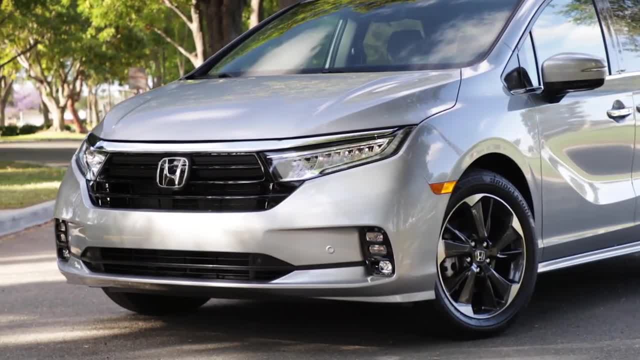 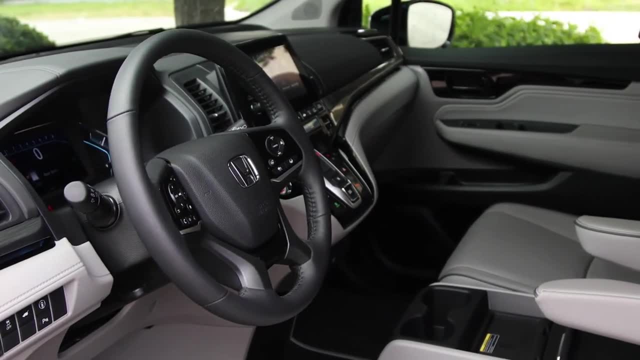 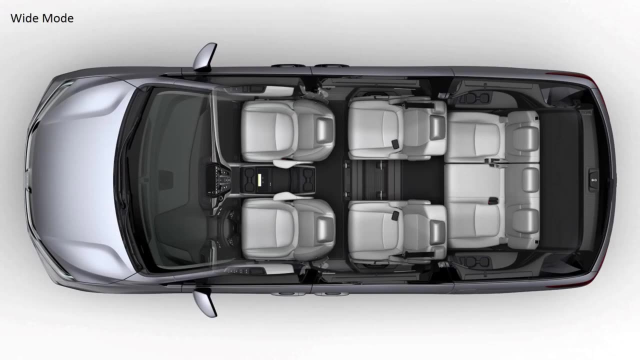 about the hybrid and the Toyota just a minute ago. I love the V6 in the Honda and I also like the minimalist approach to the interior. It's just a little cleaner, a little crisper. It rides well, It's got flexible seating, It does everything well and I like the styling of it. It looks wider. 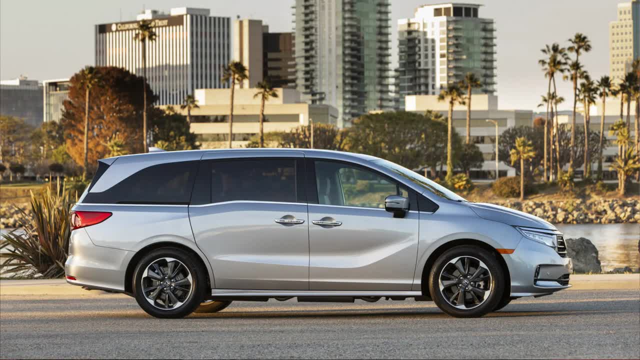 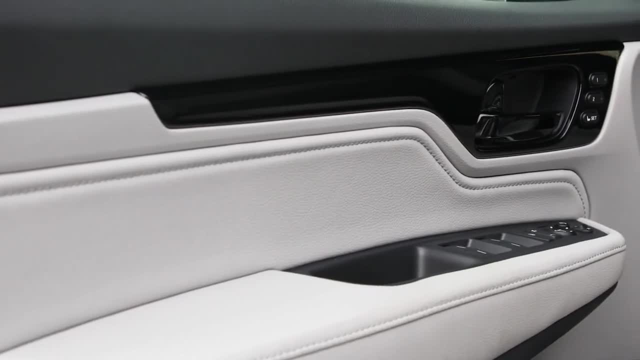 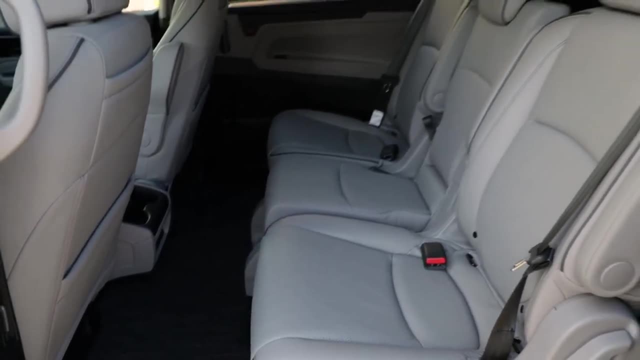 It's got that wiping bolt styling down the side. There's really nothing to dislike about this minivan. Now, if you chose the Toyota over the Honda, I'm certainly not going to get upset about it. If you chose the Carnival, I wouldn't get upset about it. If you chose the Pacifica. 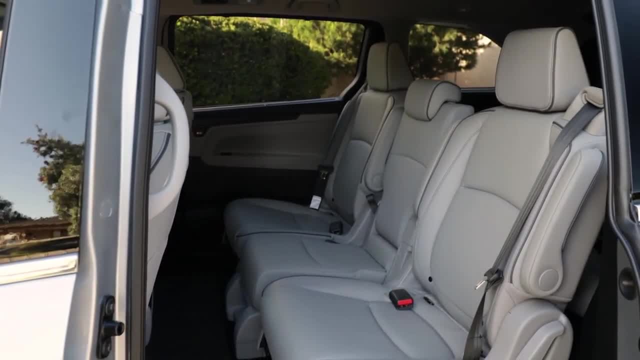 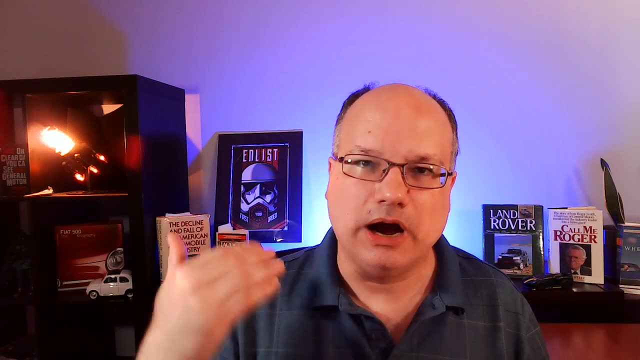 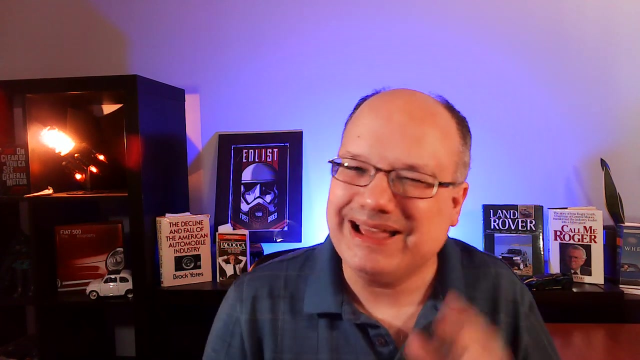 you know. fine, That's your choice. I wouldn't get upset about it, but I do think that the Odyssey is our number one choice. We've looked at these vans and ultimately is what I've told you: The Pacifica. honestly, don't trust the reliability of it and don't. 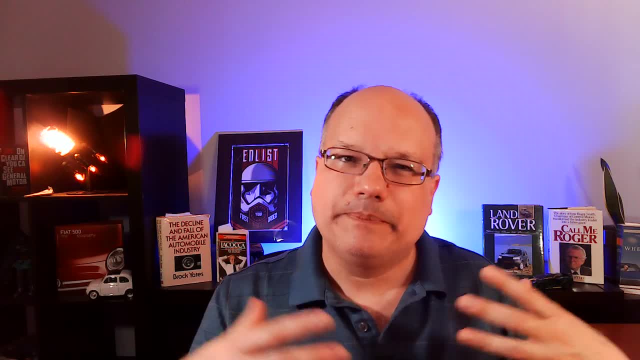 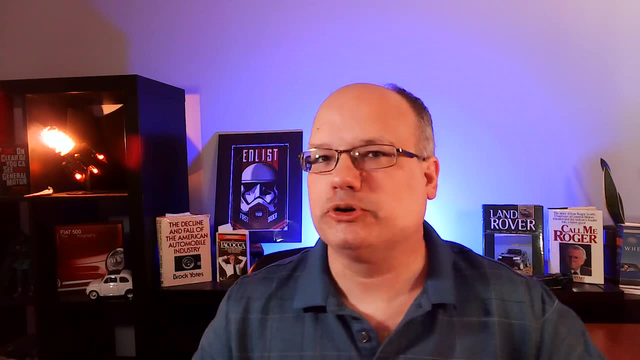 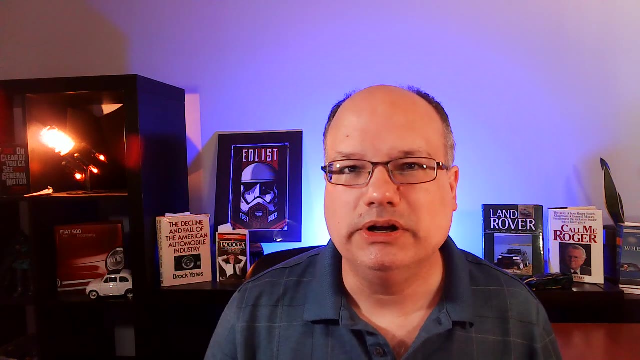 really love the styling, The Carnival, the name, what it offers for the price. is it worth it? over the top two? And then the Sienna and the Odyssey, number one and number two for us. Which one do you choose? Well, it's a matter of personal taste and the flavor of the vehicle, I got to admit. 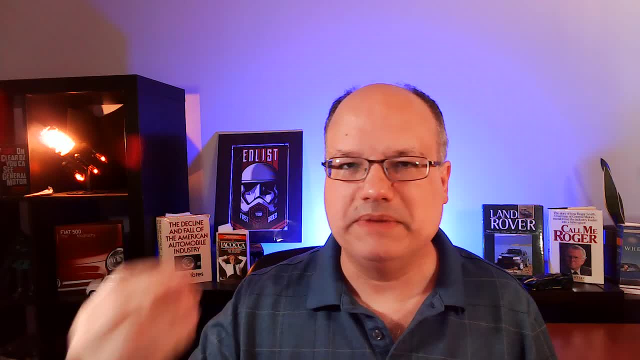 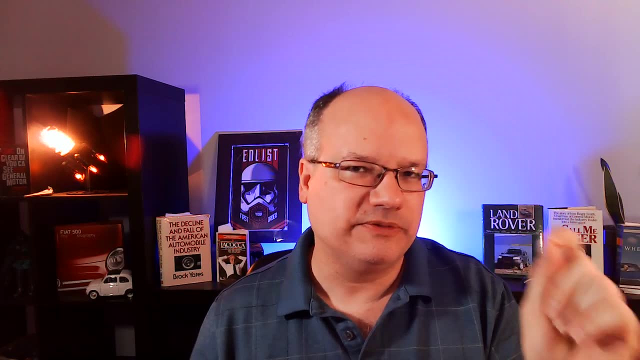 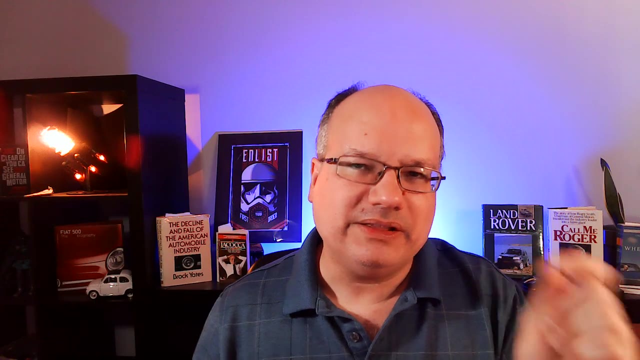 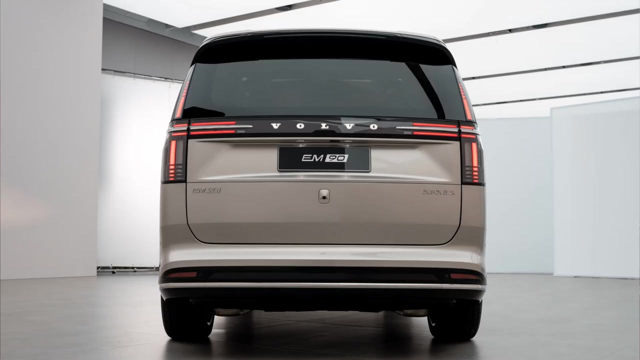 I prefer the Honda overall for its minimalist style. And that leads me to my honorable mention, which is the Volvo EM90.. Now, I mentioned this at the end because, number one, it's not available in America and they haven't said whether they're.